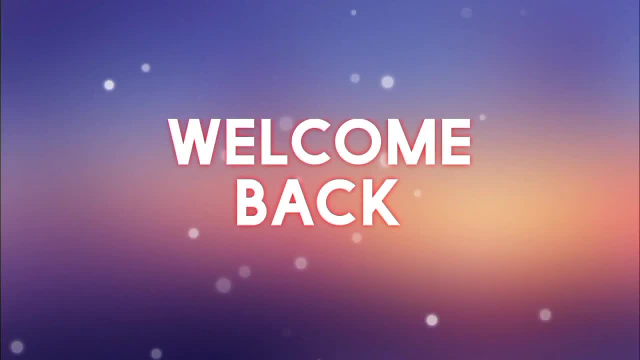 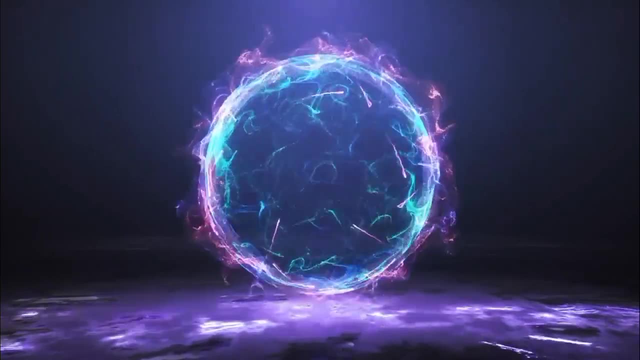 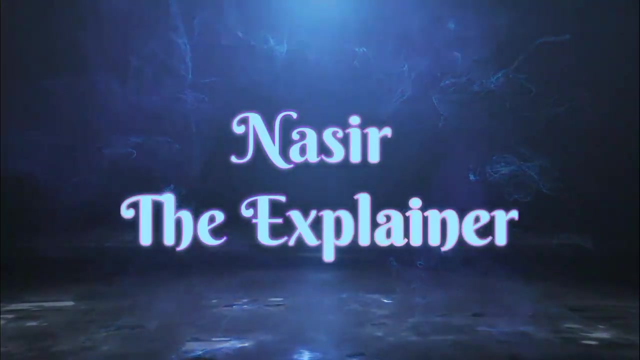 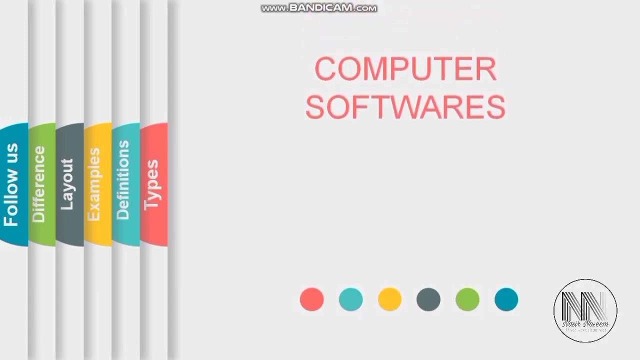 Hello everyone, welcome back to my channel, Nasser the Excellenor. I hope you all will be fine. Today we are going to talk about computer software. We will discuss the types of the software, their definitions, their different examples and their difference between the types of the computers. 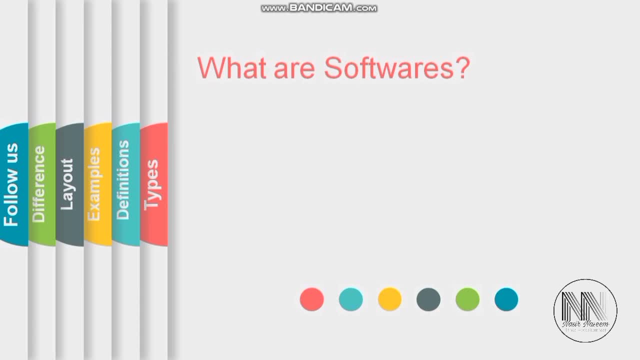 So proceed further. It is must to know what are the softwares. So computer software is the set of instructions that tells the computer hardware what to do. Or in other words, we may say software comprises the entire set of programs, procedures and routines associated with the operation of a computer system. 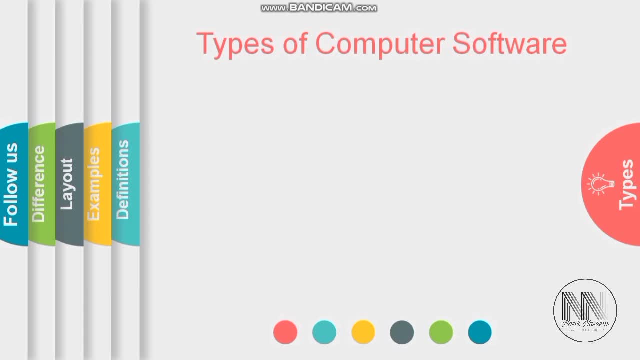 The next point is that what are the types of the computers? Computer software can be classified into three types of the. First is system software, Second is application software And third is web software, Or it may be called as web based software. These may be: 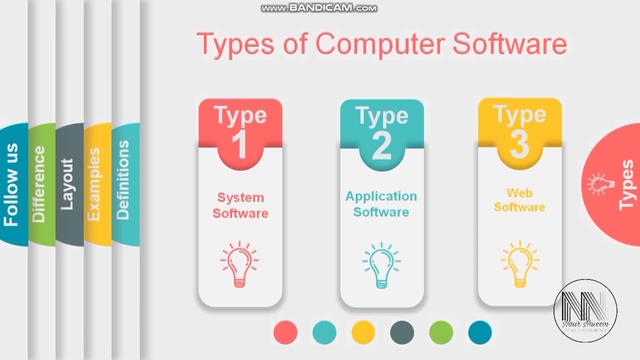 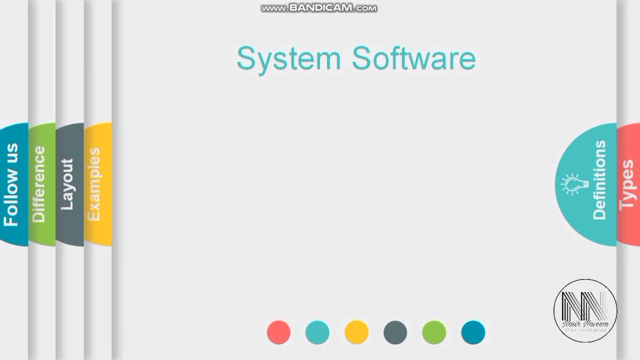 system software And these may be web-based application software. So the next point is about the definitions of these types of the computer software. So system software are the software that control a computer's internal functioning, So they can operate briefly through an operating system and also control such peripherals such as monitors, printers and storage devices which are attached to a computer system. so all these computer hardware are controlled by a system software. 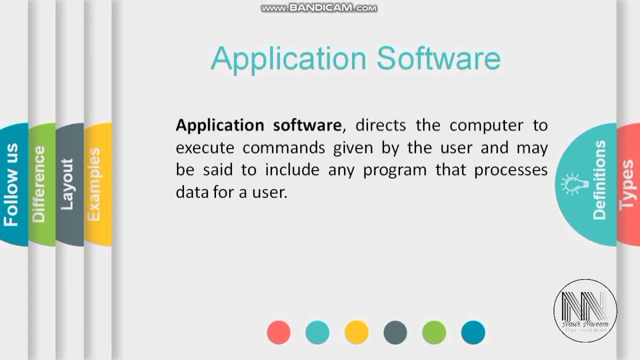 Next is application software. Application software direct a computer to execute commands which are given by a user And may be said to include any program that process a data or any data for a user. Application software can be self-contained or it can be a group of programs that run the application for the user. 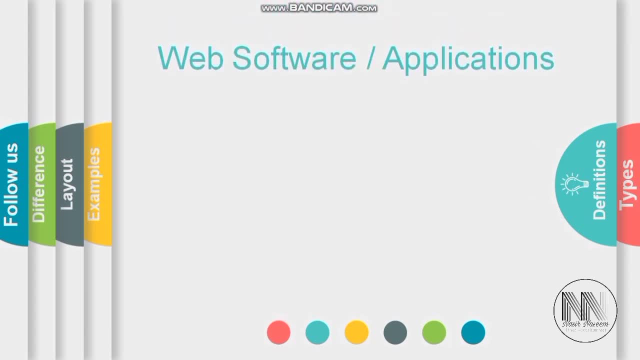 Next is Web. software Are web-based applications We have based. applications, on the other hand, only require internet access to work. They do not reply on The hardware system. also, software system software to run. Consequently, users can launch any web application from The devices that have a web browser. 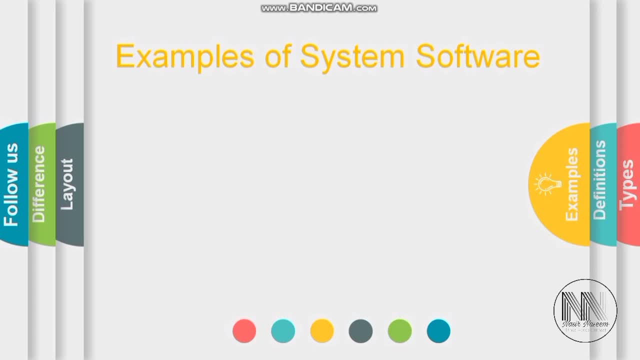 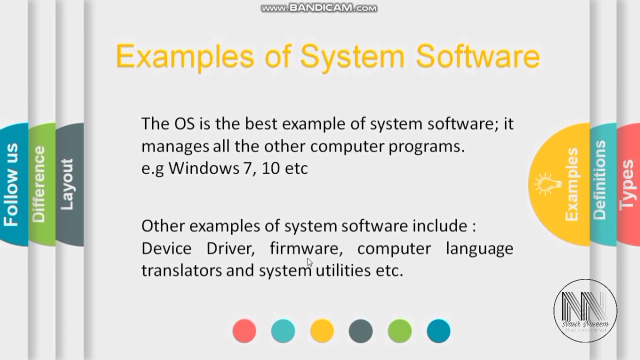 So examples of the system software. the operating system is the best example of the system software, and The examples of an operating system is Windows 7, Windows 10, Windows Vista, Linux. Some other examples of the system software are device driver, firmware, computer language translators, system utilities. Now 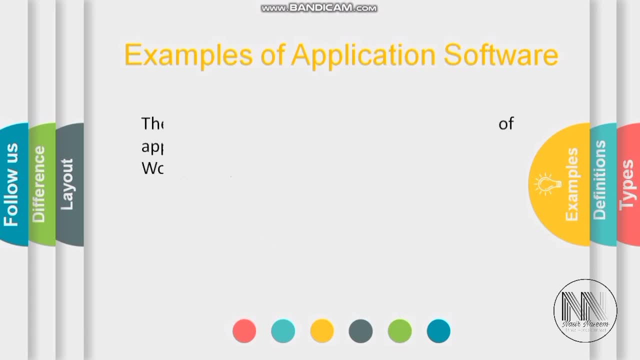 different examples of application software. So the office management is the best example of application software. it includes word, excel, PowerPoint, etc. and some other examples of the application software: that web browser, database management, inventory and payroll program and some examples of web software and which are the Web mail, very word processor, subred sheets, video and photo editing online which are based on the internet. 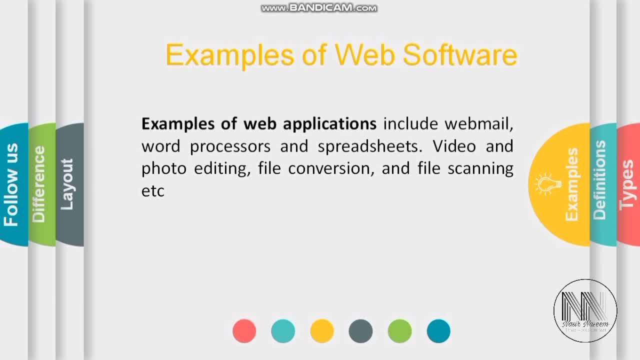 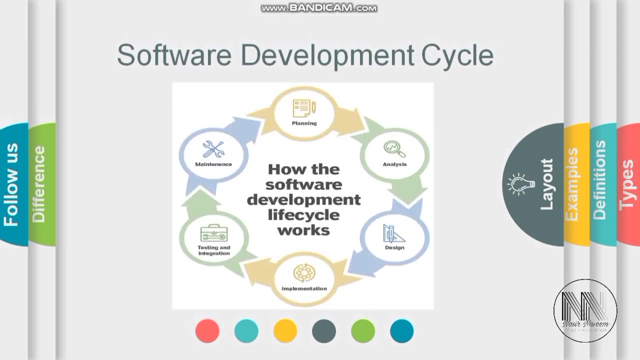 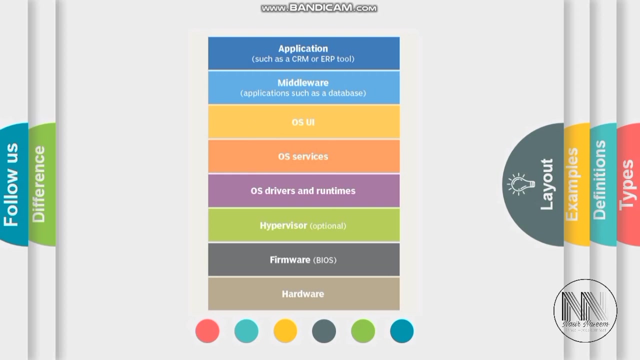 file conversion system, file scanning system, which are can be obtained through a web browser. So this is a software development cycle. There is a large number of planning, analysis, design, implementation, etc. There is a layout of the system, application and hardware of the system, computer system. So from this layout it is clearly visible that all types of the applications or softwares are